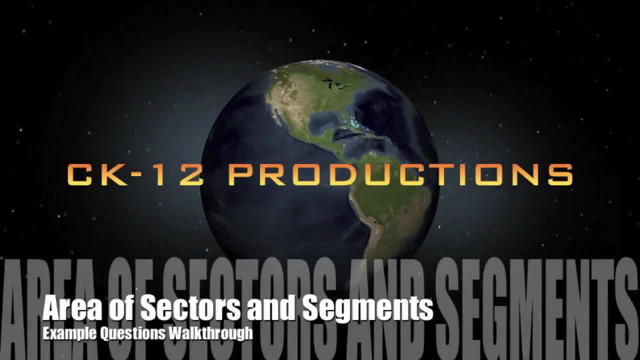 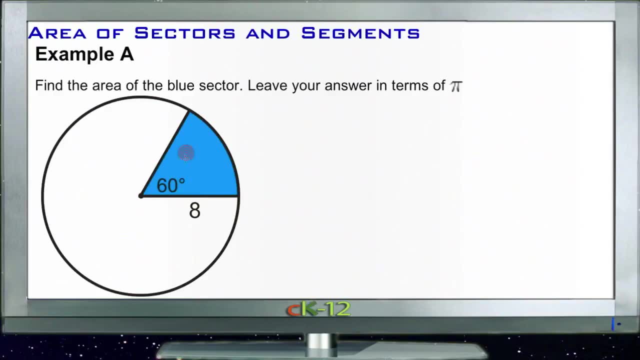 Okay. so example A asks us to find the area of the blue sector, and we're supposed to just leave our answer in terms of pi. So the first thing we need to do to find the area of this sector is find the area of the entire circle. Now we know that the radius of the circle 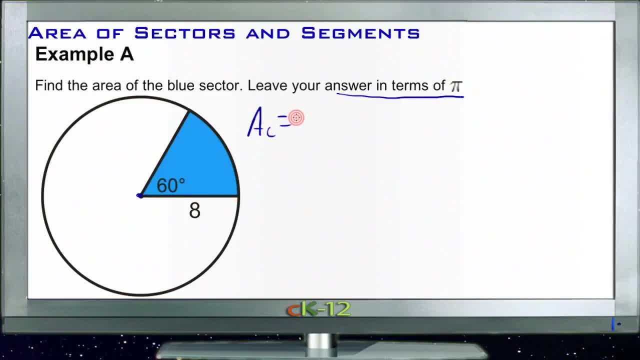 is 8 units and the area of a circle is pi times the radius squared. So if it's 8 units for the radius, then we have pi times 8 squared, or 64 pi, as the area of the circle. Now, now that we know the area of the entire circle- 64 pi- we need to find out what portion of 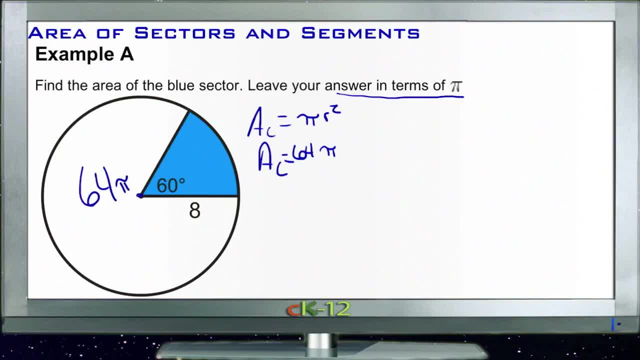 that entire circle's area we have in our little sector right here. So we take a look at the degree major of the sector. we have 60 degrees and since our sector is 60 degrees and the entire circle is 300. So if it's 360 degrees, we have 60 360ths, or 1 sixth of the entire circle. So if the 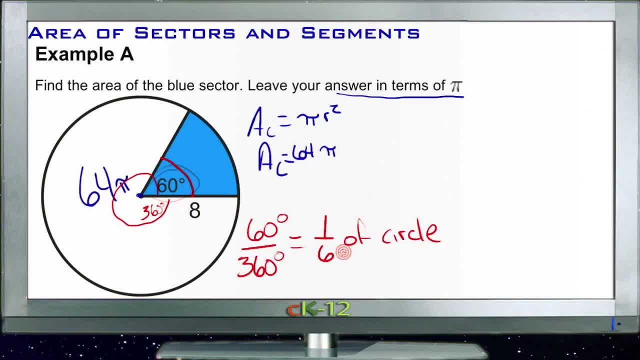 area of the entire circle is 64 pi units and we have 1 sixth of that area. then we have 1 sixth of 64 pi And if we multiply or divide 64 by 6, we get about 10 and 2 thirds. So we get about 10 point. oops, that was a bad 0,, sorry, 10.66. 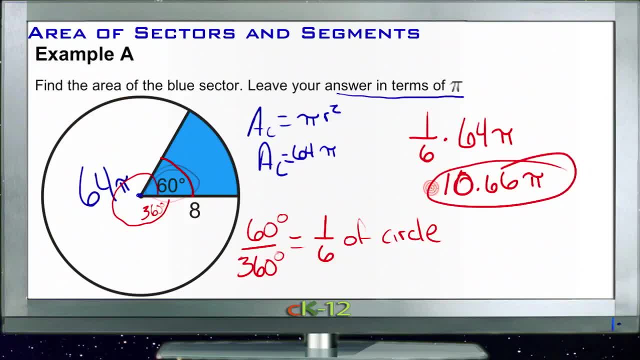 pi units as the area of our little sector. Yeah, 1 sixth of the area of the entire circle. and the area of the entire circle is just the radius squared times pi. That's it. Let's take a look at the next one. 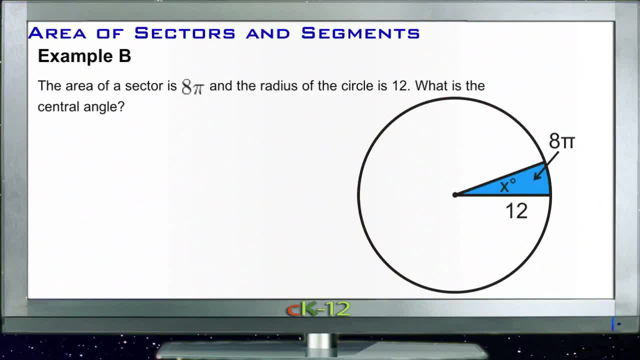 Example B: The area of the sector is 8 pi and the radius of the circle is 12.. What's the angle? Huh, so now we're going the other way. Now we know the area of this little segment right here. we don't have to. 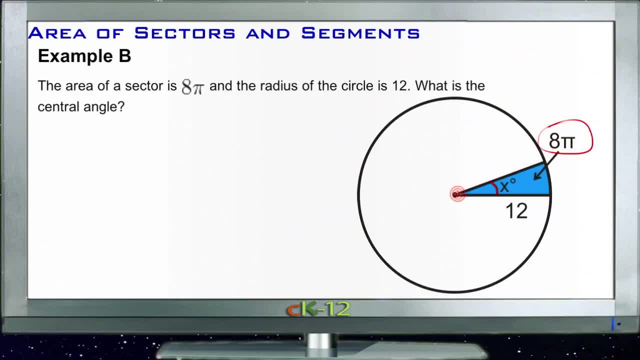 calculate it. We don't know the area of the whole circle, but we do know the radius of the circle. So if we find the area of the circle real quick here, we know that it is going to be pi r squared, so its going to be 12 squared times pi, or. 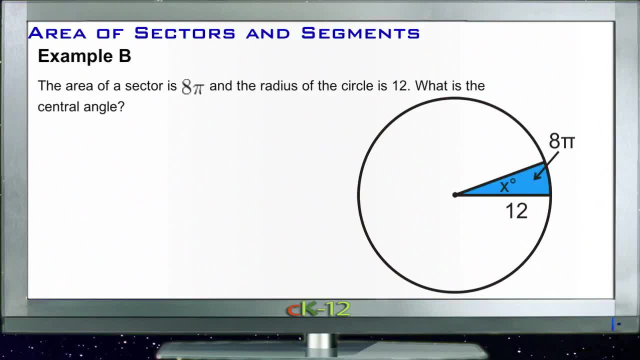 Example B: The area of the sector is 8 pi and the radius of the circle is 12.. What's the angle? Ah, so now we're going the other way. Now we know the area of this little segment right here. we don't have to calculate it. We don't know the area of the whole circle. 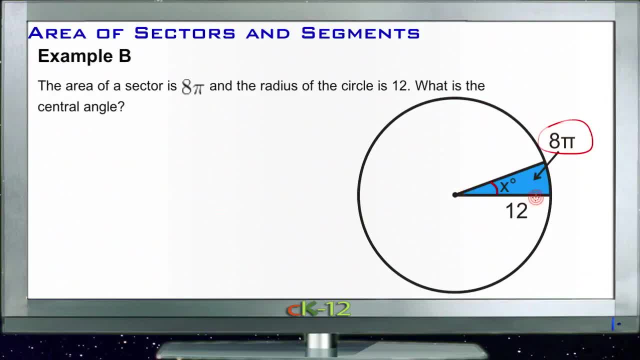 but we do know the radius of the circle. So if we find the area of the circle real quick here, we know that it's going to be pi r squared, so it's going to be 12 squared times pi, or 144 pi for the whole circle. we have 8 pi. so if what we have is 8 pi out of 144 pi, 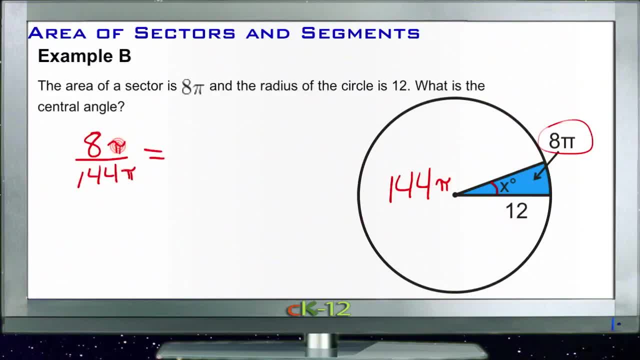 what we want to know is: by the same comparison or in the same ratio, what's x degrees out of the total number of degrees, which is 360? so we have a proportion. the area of the little segment compares to the area of the entire circle, the same way that the degree measure inside compares to the 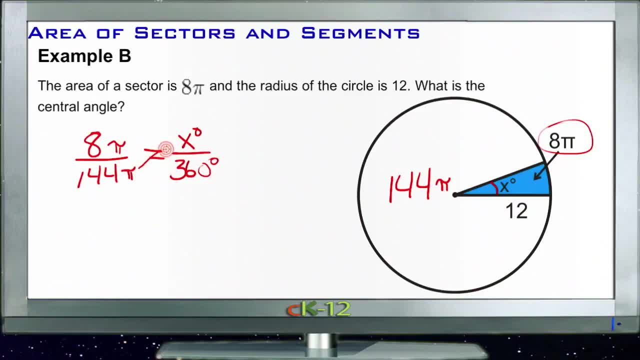 degree measure of the entire circle. so now we can just multiply and we get 8 pi equals. in fact we can just cancel the pies right at the beginning, don't worry about them at all. 8 equals 144 X. I got a cross multiply. sorry about that. let's go. 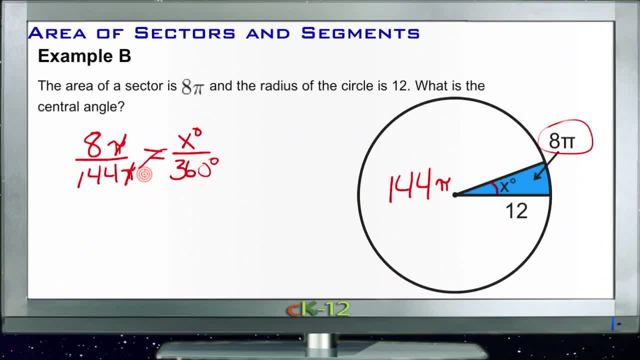 to the back of that up, we'll go ahead, and we'll go ahead and cancel our pies anyway, but we'll cross multiply, so we'll do 144. X is equal to 8 times 360, 360 times 8, 28, 80, 28, 80. okay. 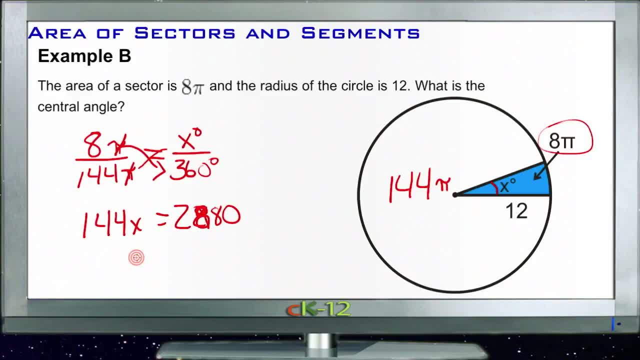 and then we divide both sides by 144 and we get 20. so 20 degrees represents the degree major of our little segment right here out of the 360 that represents the entire circle. the same way that 8 pi represents the area, the segment, the same. 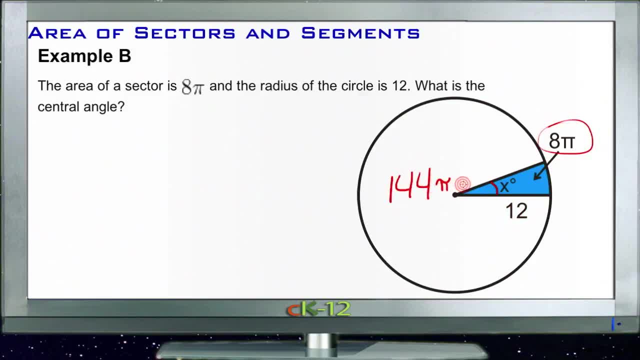 144 pi pi. Here we go the whole circle. we have 8 pi. so if what we have is 8 pi out of 144 pi, what we want to know is, by the same comparison or in the same ratio, what's X degrees out of the total number of degrees, which is 360? so we have a proportion, the area. 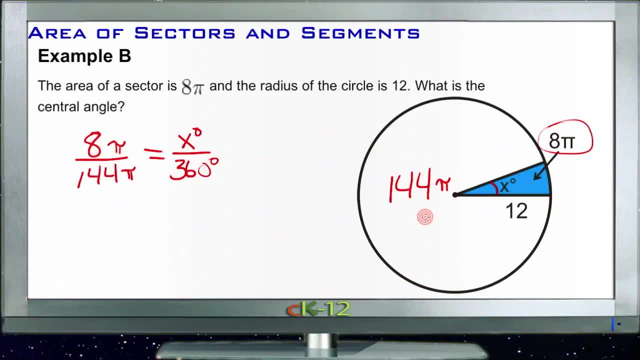 of the little segment compares to the area of the entire circle, the same way that the degree measure inside compares to the degree measure of the entire circle. so now we can just multiply. can we get 8 pi equals? in fact, we can just cancel the pies right at the beginning. now we're about them at all: 8 equals. 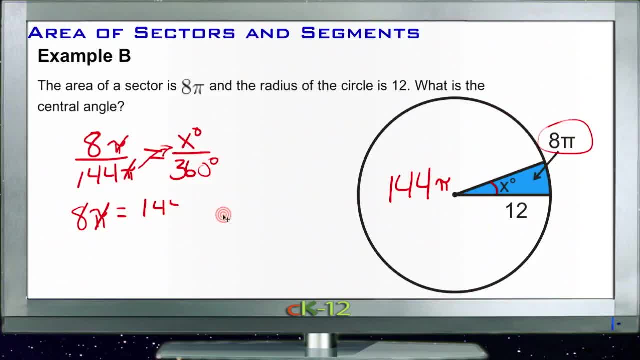 444 X. I got a cross multiply. sorry about that. let's go back that up. we'll go ahead, and we'll go ahead and do that again and cancel our pies anyway, but we'll cross multiply, so we'll do 144. X is equal to 8 times 360, 360 times 8, 28, 80, 28, 80. okay, and then we divide both sides. 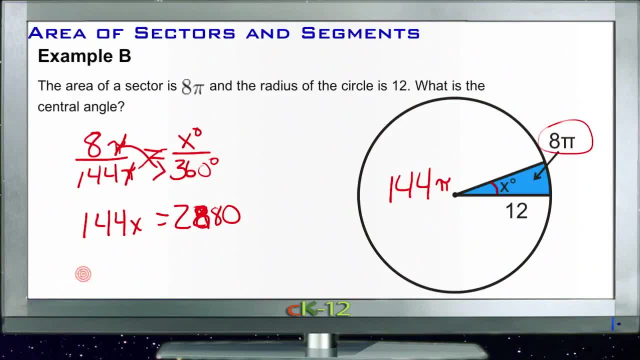 by 144 and we get 20. so 20 degrees represents- that agree- major of our little segment right here. out of the 360 that represents the entire circle, the same way the 8-pie represents the area of the segment, the same way 144pi represents the area, the 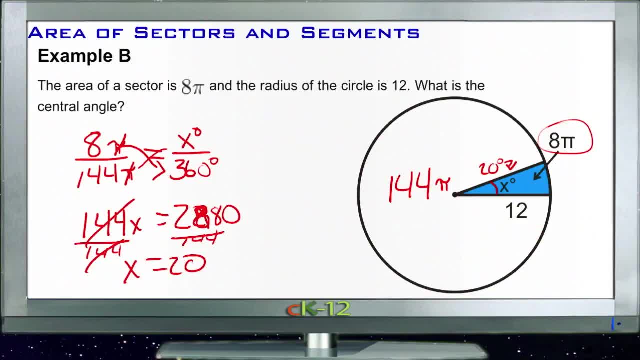 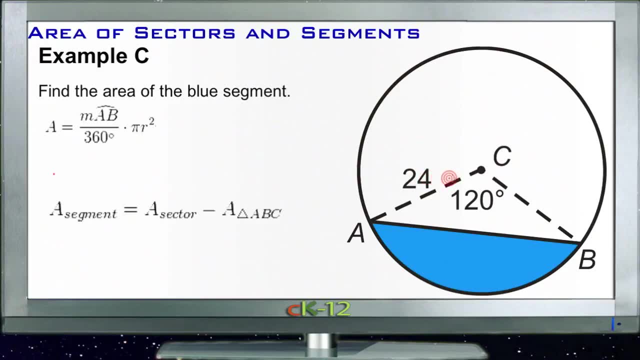 whole circle. cool, great example. see alright, for example. see here we need two women. you do a two-step process. the first thing we need to do is find the area of of the sector that incorporates the segment we're looking for, the actual area of. Our goal is to find the area of just this blue portion here. but the first thing we 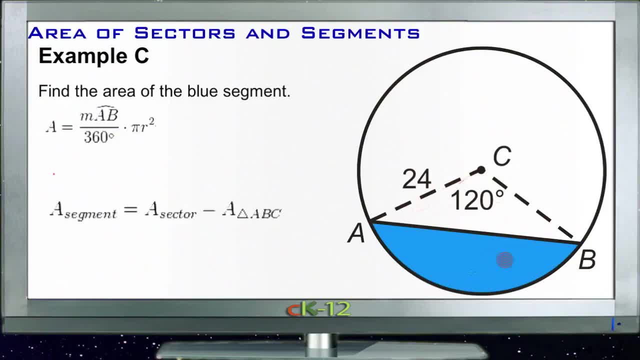 can find the area of more easily is the area of this entire sector here that's incorporated by this 120 degrees. So what we need to do is find the area of the full circle and then take one third of it, since 120 degrees is one third of a circle- to find the area of that entire sector down. 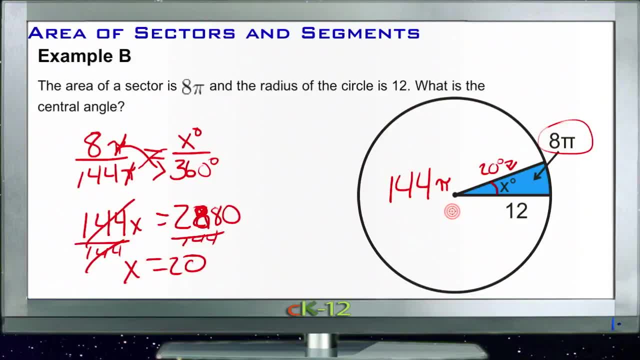 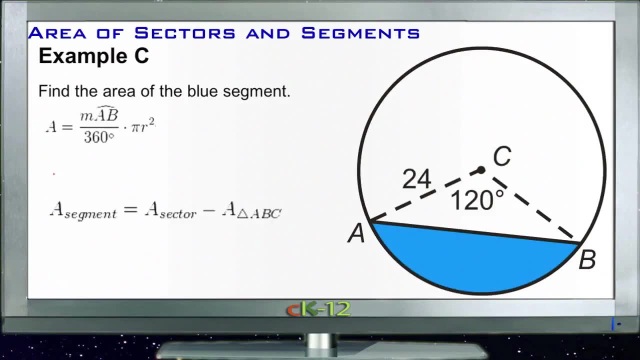 way, 144 pi represents the area, the whole circle. cool, alright, let's try example C. alright, for example. see, here we need to do a two-step process, the The first thing we need to do is find the area of the sector that incorporates the segment we're looking for, the actual area of 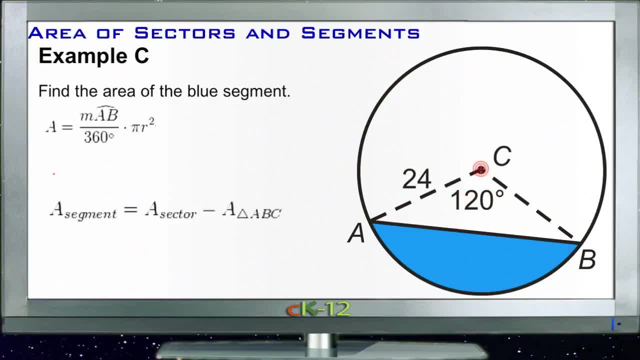 Our goal is to find the area of just this blue portion here, But the first thing we can find the area of more easily is the area of this entire sector here that's incorporated by this 120 degrees. So what we need to do is find the area of the full circle and then take one third of 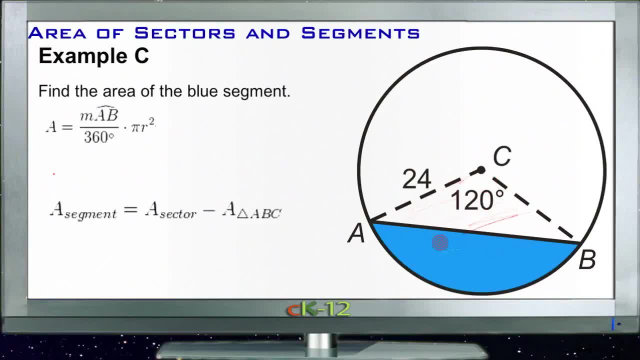 it, since 120 degrees is one third of a circle, to find the area of that entire sector down here. So let's start with that. The area of the circle is going to be 24 squared pi units. right, because it's pi r squared. 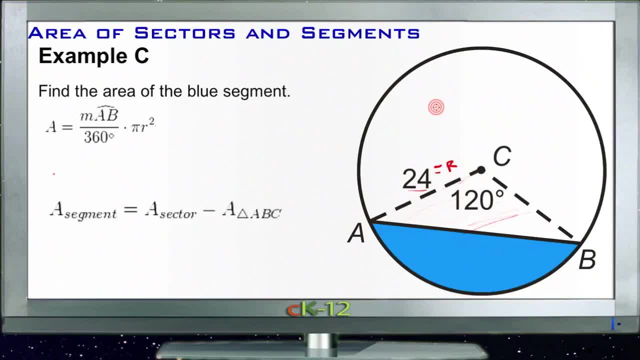 24 is our radius. So the area of the circle, 24 squared 24 times 24, is 576.. So the area of the whole circle is going to be 576 pi. square units, Square units. Okay, Now our sector down here is just one third of that, because it's only 120 degrees out. 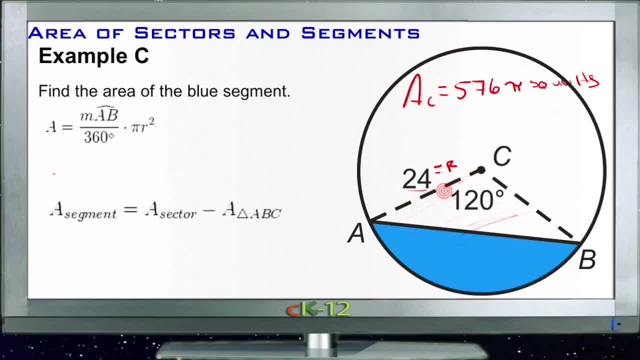 of the 360 degrees. So if we divide our 576 by 3, divide by 3, then our area of our sector is going to be 192 square units. Yeah, So we took the major of the sector over 360.. 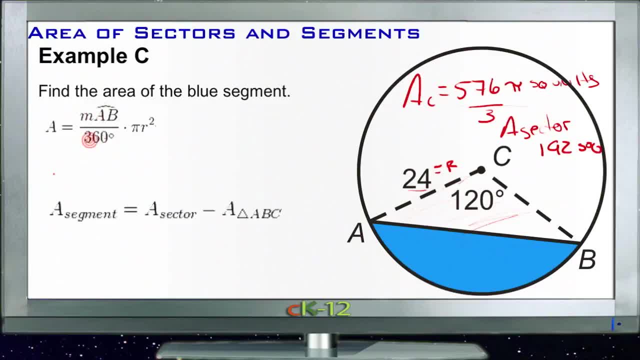 That was our 126.. 20 over 360.. So we had one third of our total. Pi r squared is the area of the whole circle, So one third of 576 gave us 192 square units. yeah, So 192 square units is the area of a segment of the sector. okay. 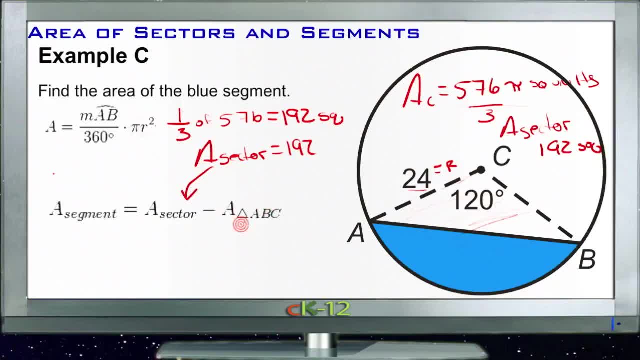 So now we know the area of the sector, We need to find the area of the Triangle ABC Now to find that we've got to learn something more than just one side. We do know that it's 120 degrees all the way across the top of this thing. 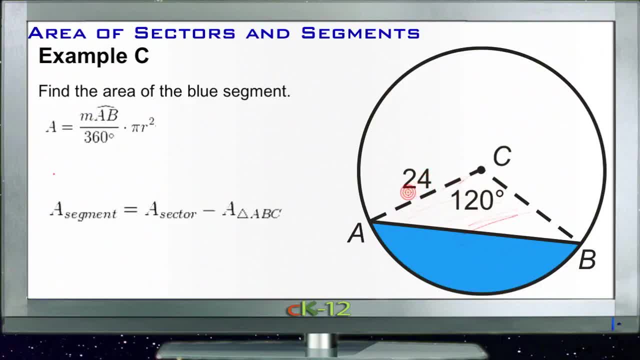 here. So let's start with that. So the area of the circle is going to be 24 squared pi units, right, because it's pi r squared. 24 is our radius. yeah, So the area of the circle, 24 squared 24 times 24, is 576, so the area of the whole. 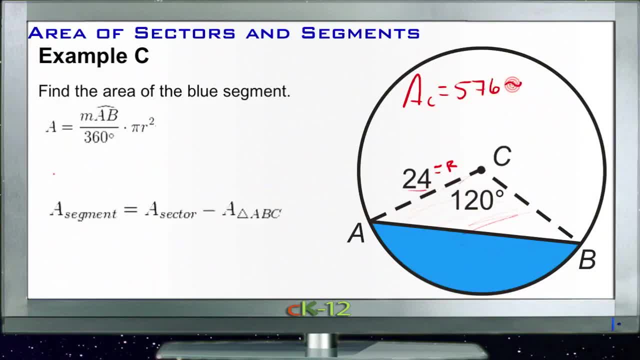 circle is going to be 576 pi square units, square units. Now, our sector down here, It's just one third of that, because it's only 120 degrees out of the 360 degrees. So if we divide our 576 by 3, divide by 3, then our area of our sector is going to be: 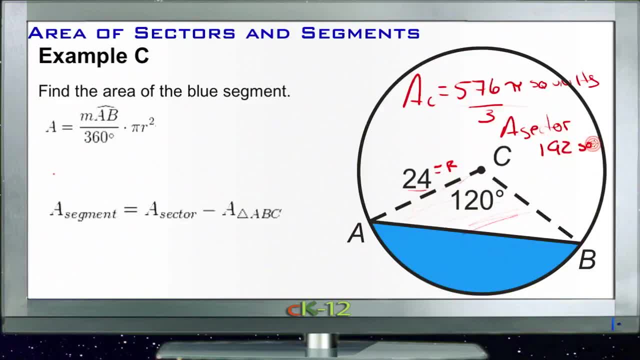 192 square units. yeah, So we took the major of the sector over 360, that was our 120 over 360. So we had one third of our total. pi r squared is the area of the whole circle, so one third. 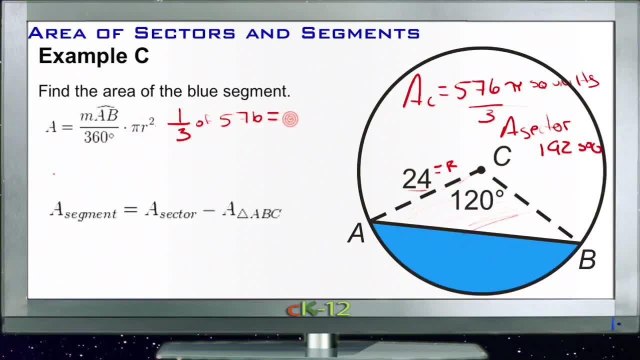 of 576 gave us 192 square units. yeah, So 192 square units is the area of a segment of the sector. okay, So now we know the area of the sector. We need to find the area of the triangle ABC Now, to find that we've got to learn something more than just one side. 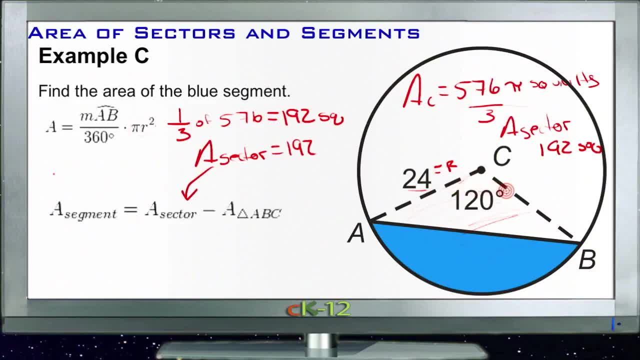 We do know that it's 120 degrees all the way across the top of this thing. Well, if we were to split this thing in half, right down through the middle, right here, and form a 90 degree angle here and here, then that would also split this upper angle. 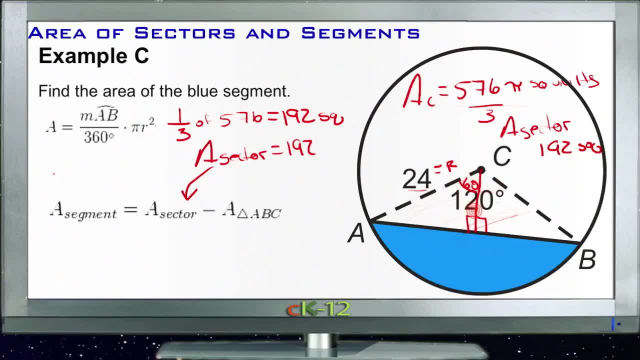 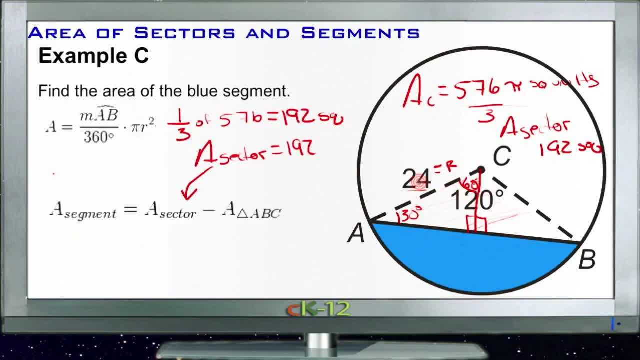 90. And on a 30,, 60, 90 triangle this side over here would be half of the hypotenuse. so this side over here would be 12 units and the side down on the bottom would be 12 roots. 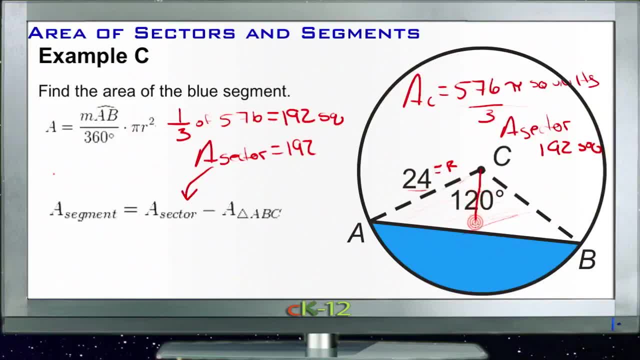 Well, if we were to split this thing in half right down through the middle, right here, and form a 90 degree angle here and here, then that would also split this upper angle in half and that would give us a 60 degree angle right here, right. 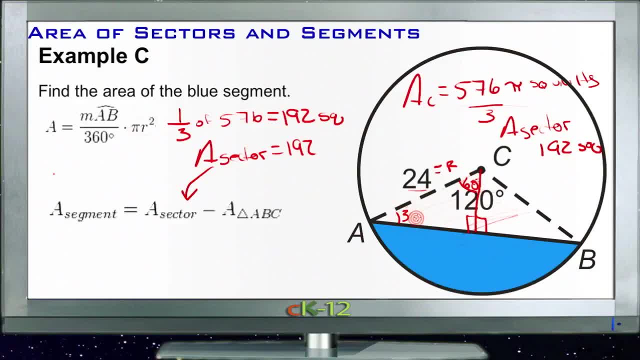 Well, if that's a 60 degree angle, then this is a 30 degree angle, because this is a 90. Now we've got our 30,, 60, 90, 20.. Triangle again right, And on a 30,, 60, 90 triangle, this side over here would be half of the hypotenuse. so this: 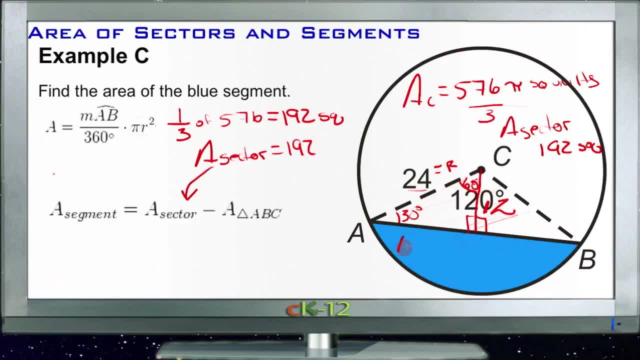 side over here would be 12 units, and this side down on the bottom would be 12 roots of 3 units, right? So if it's 12 roots of 3 from here to here, then it's 24 roots of 3 from here to here. 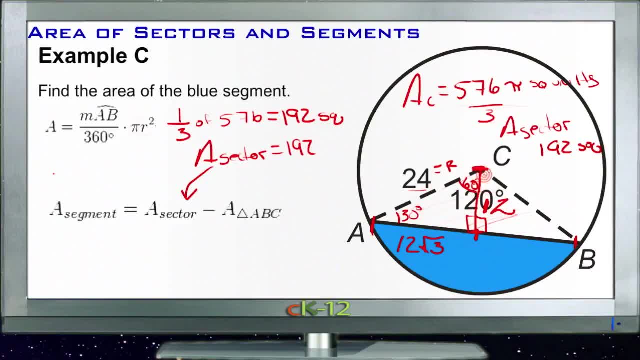 and it's 12 units from here to here. So now we have a triangle. we're trying to find the area of. We do 1 half base times height. right, The whole base is 12 times 2 roots of 3.. 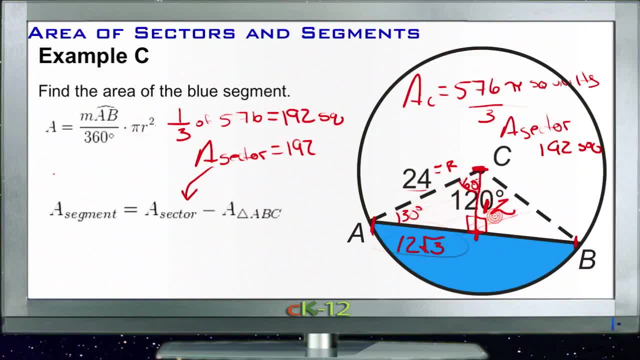 We only want 1 half. so we're just going to stick with our 12 roots of 3, and we're going to take that times 12.. So we're going to have 144 roots of 3 as the area of our triangle. 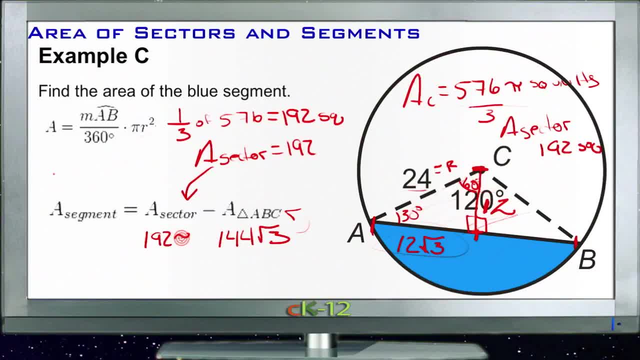 The area of our sector was 192 pi. So we're going to have 192 pi minus 144 roots of 3, and if we run all that through a calculator, 192 times 3.143.. 4159 gives us 603.19 minus, and then 144 times the square root of 3 is 249.41.. 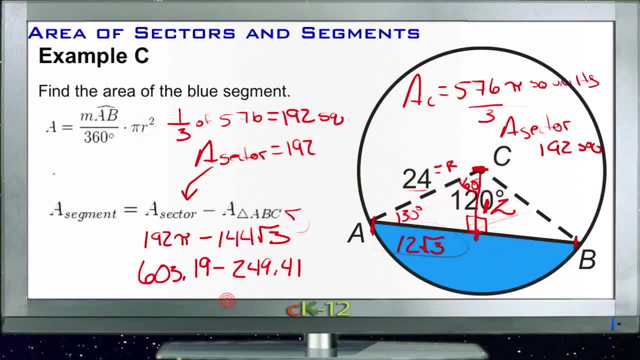 So if we then subtract those two, 603.19 minus 249.41.. We get a square root of 3.. Okay, 249.41.. We get 353.78,, 353.78, 353.78 as the area of just our little segment down here, that's. 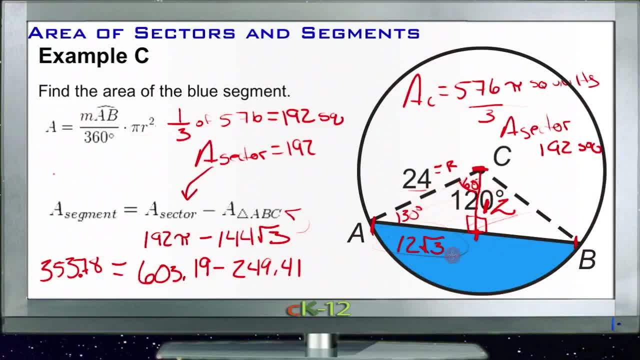 highlighted in blue And that one was a little bit of math. Hmm, kind of cool All done.